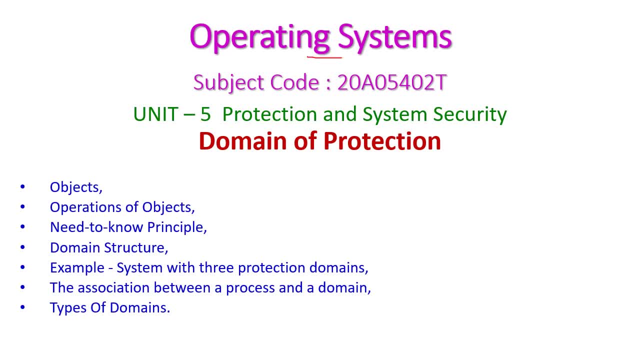 Hello friends, welcome to today's operating system class and in this class we will see the domain of protection that will come under fifth unit and in today's class we will see what is objects and operations of objects and need to know, principle, domain structure and we will see some examples and the system with three protection domains. then we will see the association between process and domain and finally we will see the types of domains. 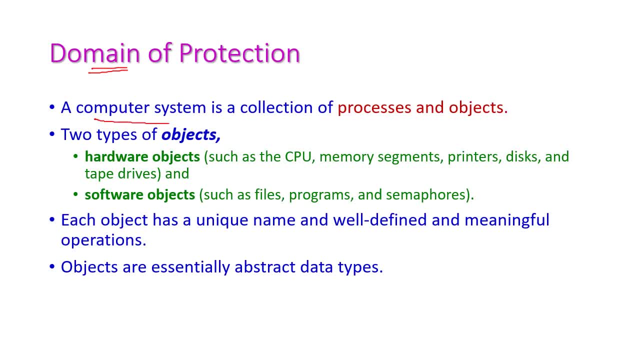 Domain of protection Here. our computer system is a collection of processes and objects. First let us see object. Here we are having two types of object. First one is hardware object and second one is software objects. So hardware objects- there are CPU, memory segments, printers, disk and tape drives, etc. All physical components will come under hardware objects And when come to software objects, all the software, that is, program components, will come under hardware objects. 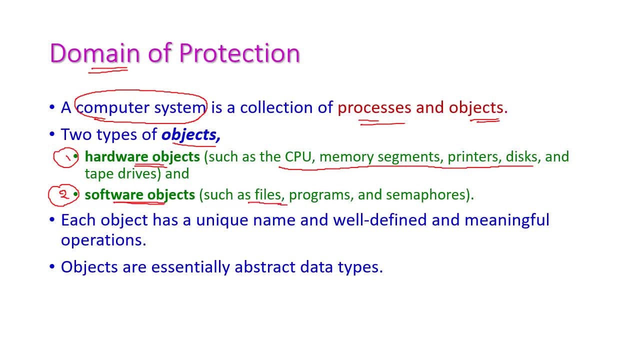 And when come to software objects, all the software, that is, program components, will come under software objects. Here files, programs, some of us, and these are some of the example of software objects. Here each object has unique name. By using the name only we can identify the objects. and the objects are having well defined and meaningful operations. So the operations will define the purpose of that. objects, Okay, and objects are essentially abstract data type. 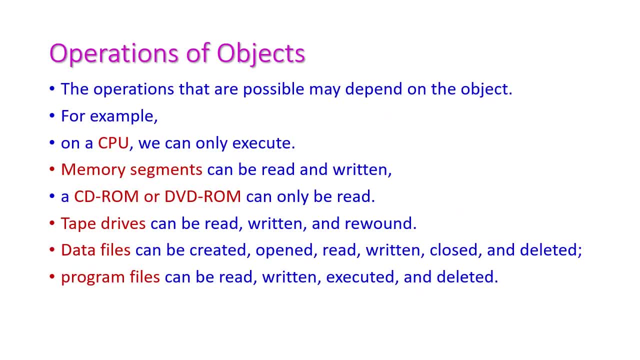 Next, let us see the operations of objects. So, based on the objects, the operations will be different. For example, a CPU, CPU can only execute some programs And memory segments. memory segments: we can store the data and the data will be read or write. 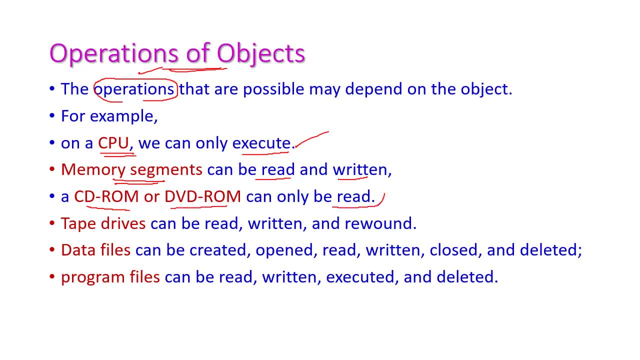 When come to CD-ROM, DVD-ROM, we can only read the data which are stored in that CD-ROM or DVD-ROM. Tape drives can be read or write, Read, written and rewound- And data files. data files can be created, opened, read, write, close and deleted. So these are operations that will be belongs to the data files. 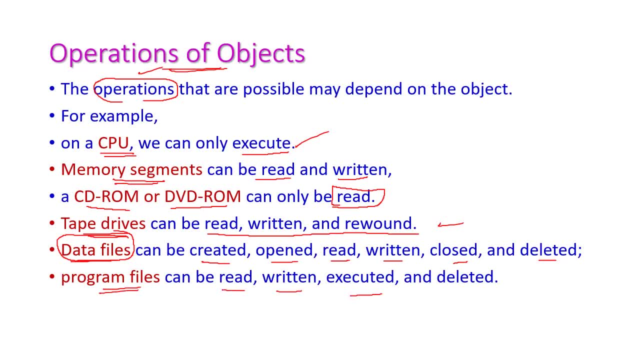 When come to program files, we can read, write, execute and delete, So the program files will be executed. So for a particular purpose we have create the program file, But for executing this program file we can use this data file. So back to CD-ROM. 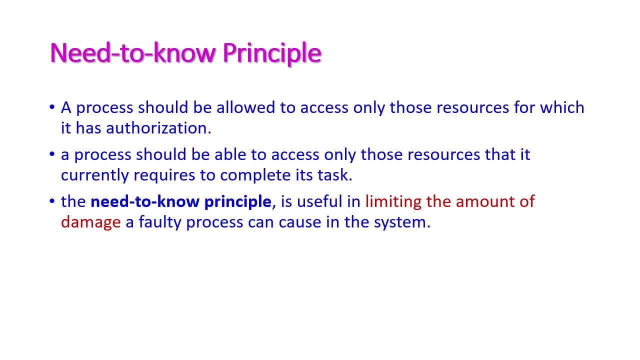 So back to CD-ROM. So back end data will be stored in data files. And next let us see this need to know principle Here: the process should be allowed to access only those resources which are authorized. Okay, The process is allowed to use only the authorized resources to complete its current task. 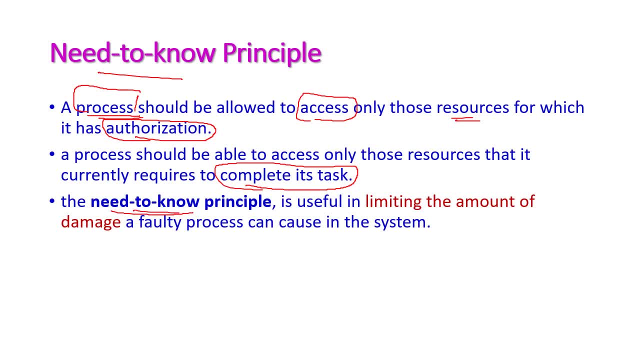 Okay, And here the need to know principle is very much helpful for limiting the amount of damage, That is, the hardware damage or the resource damage a faulty process can cause in the system Because the process is allowed to access only the authorized resources. then if there is any fault, access only this particular resource will get damaged and that will not affect all the other resources. 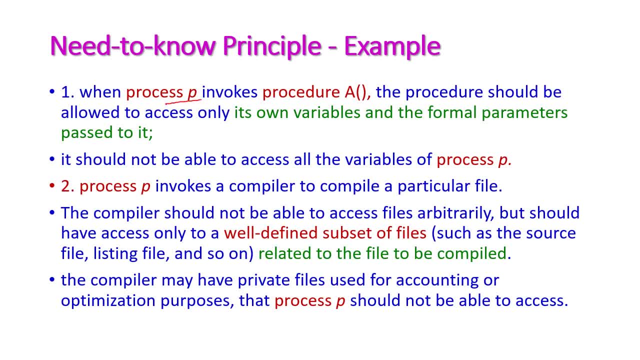 And now let us see some examples Here. the process P invokes a procedure A. Okay, A is here. Okay, This is A. Now the process P. try to call this particular procedure. Now, the procedure should allow only the own variables and the formal parameters. 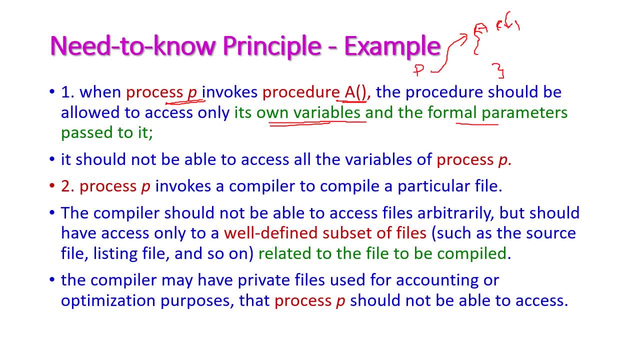 Okay, The formal parameter will be here and the local variables will be declared inside the procedure. Okay, Now the process should allow only these variables. Okay, This is a first situation. And And when come to second example, the process P invokes a compiler to compile a particular file. 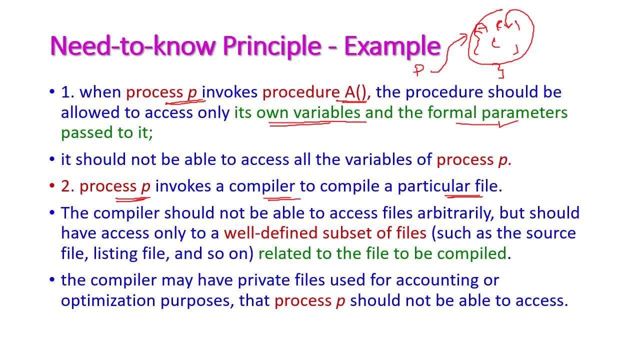 Okay, Now the process is going to compile a particular file. Here the compiler should not able to access all the files, But the compiler can execute only the file which procedure, that is, this process is going to given. Okay, That is only well defined subset of files. 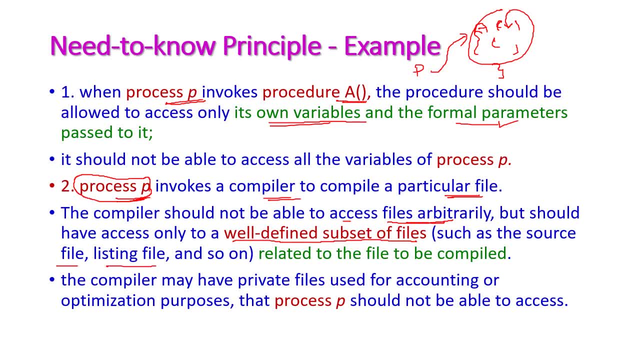 Such as Source file, Listing file And so on. That is, which is the file will belongs to this particular process That only the compiler can execute. That is the file related to be compiled for process P. The compiler may have so many private files. 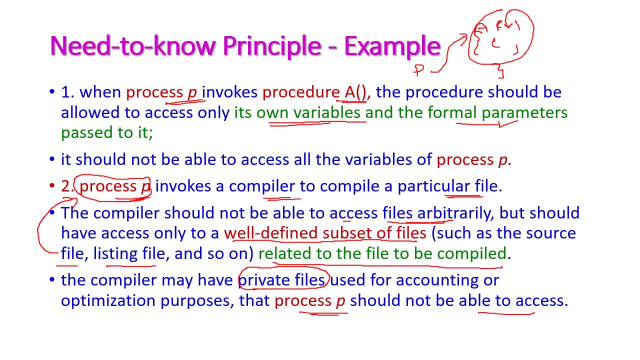 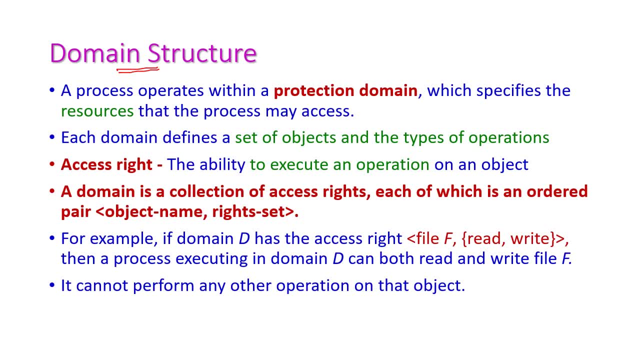 But The process should not be able to access all the files. Next, let us see the domain structure. The domain contains the process, The objects and the access rights. Okay, When come to process, It operates within the protection domain And which specifies the resources that the process may access. 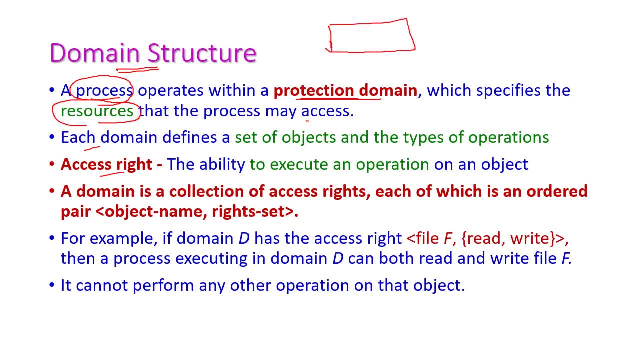 That is, within a domain. we are having so many resources And the process should execute only inside the domain with the given resources. Okay, Next, The domain defines the objects And the type of operations Which are associated with these objects. And third one is access rights. 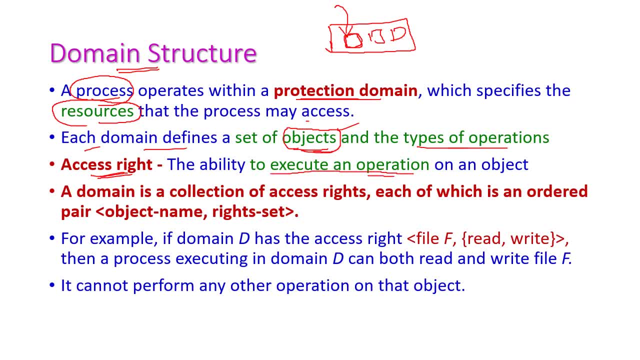 That the ability to execute an operation on that object- Okay, Which are the operations should be performed on this object? is called as access right. Okay, Now Let us define this domain with this information. Okay, Domain is a collection of access rights. 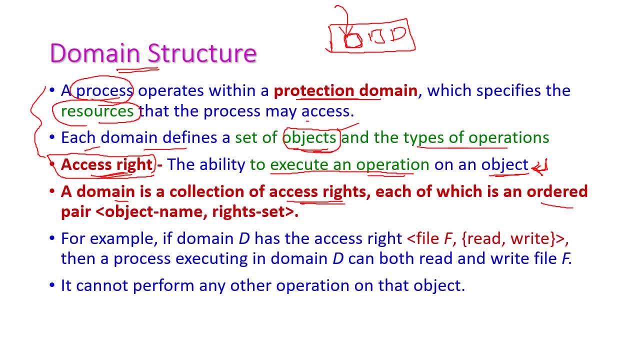 Each of which is an ordered pair. Ordered pair of domain objects. Domain object and rights set. Domain object and rights set. Okay, So this is the definition of domain. Let us see example. If domain D has access rights of what is this object name? 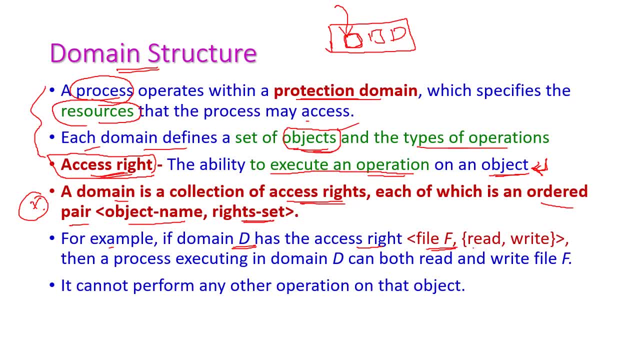 Object name is file here. What are the access right here? Read and write. That means the process executing in the domain can read or write this particular file And it cannot perform other operations on that object. That means the process cannot delete any content in this file. 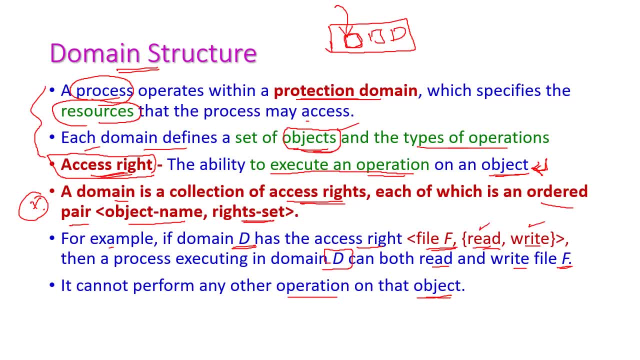 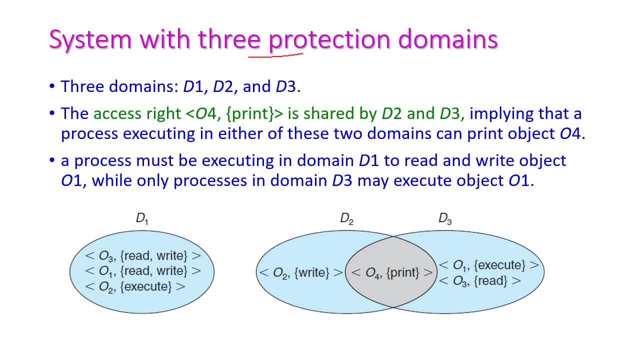 It can only read or write. Okay, This is called as access rights. Let us see another example: A system with three protection domains. Here we are having three domains: Domain 1. Domain 2. And domain 3.. Domain 1 contains three objects. 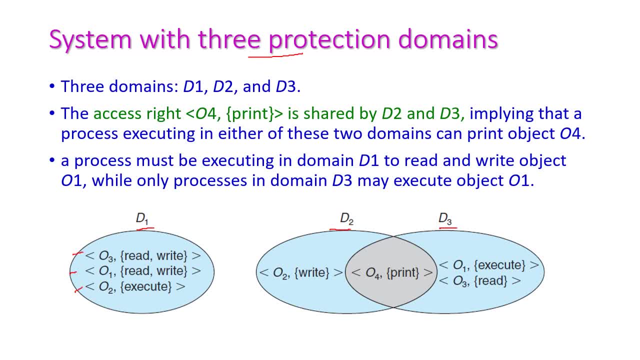 Object 1., Object 2. And object 3. With the given access rights. Okay, Object 1 will be read and write, Object 2 should be executed alone And when come to object 3, read and write will be possible in domain 1.. 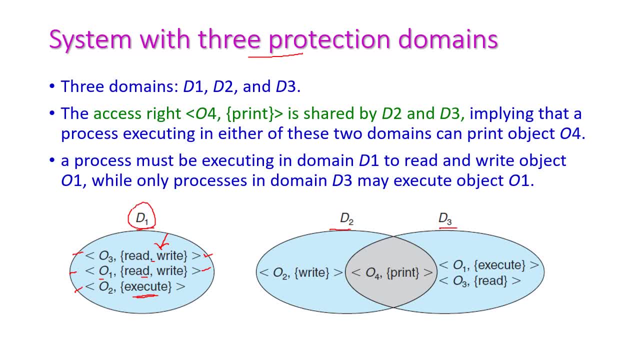 Okay, When come to domain 2 and domain 3. Object 4 is allowed to print for both domain 2 and domain 3.. Okay, And here the object 1 is allowed only read and write in domain 1.. But the object 1 is not allowed to print. 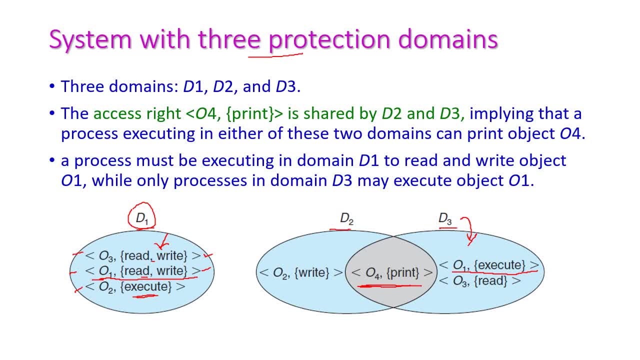 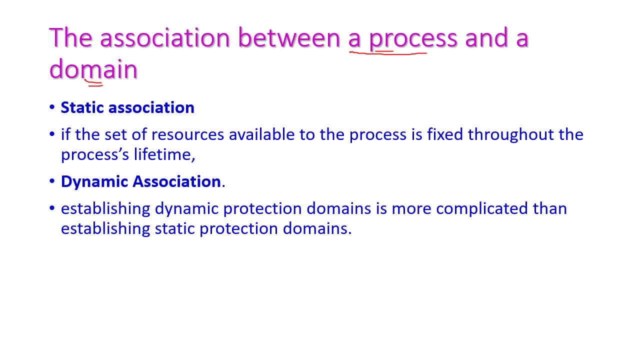 Okay, Object 2 is allowed, executed in domain 3.. Okay, Here, when come to object 2.. Object 2 is only executed in domain 1.. But the right access is given for domain 2.. Right, With this information, let us try to associate between the process and the domain. 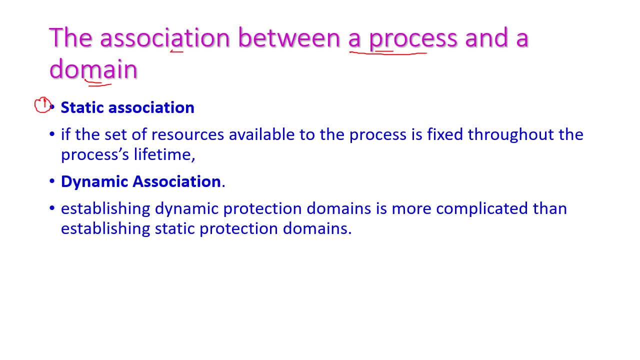 Here we are having two types of association. First one is static and second one is dynamic. Okay, Static is constant, That is fixed. That means the set of resources which are available for the process is fixed throughout the lifetime of this process. Okay, 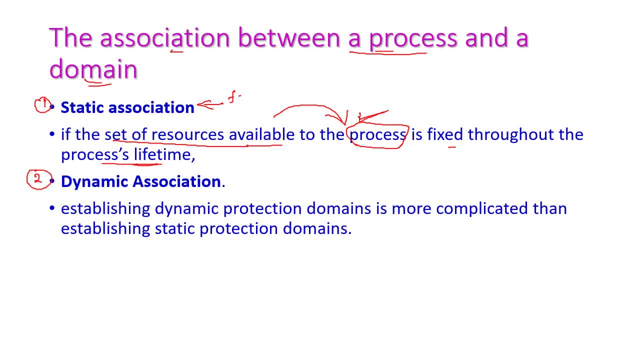 These resources will be fixed for this process throughout this process lifetime. When come to dynamic, this is not possible because the dynamic protection is more complicated when compare to static protection. That is, whenever the process required a particular process And we need to allocate this process, that should not be affect the other resources. 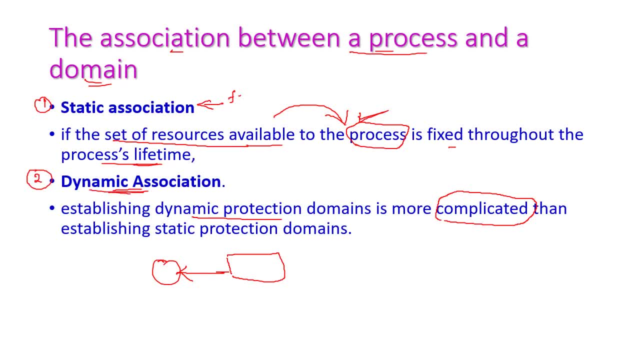 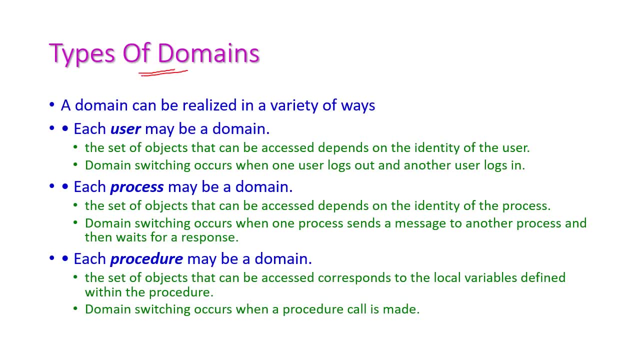 or other process. Hence the dynamic association is very, very complicated when compare to static association. And next let us see the types of domains. Here, broadly, we are having three different types of domain. First one is: user may be a domain And each process may be a domain. 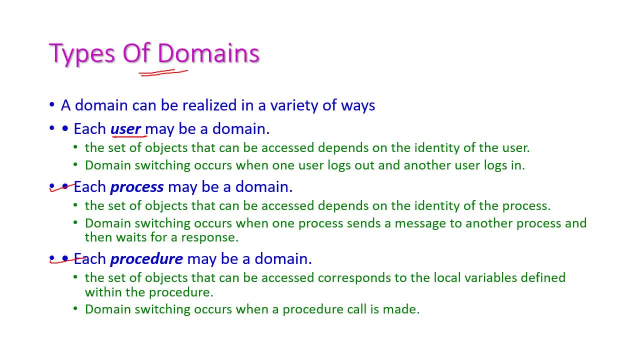 Okay, First let us see the user domain. Okay, Here the set of objects that can be accessed depend on identity of the user. Okay, When the domain switching will happen? the domain switching will occurs once the user log out the system and another user logs in. then the domain switching will happen.